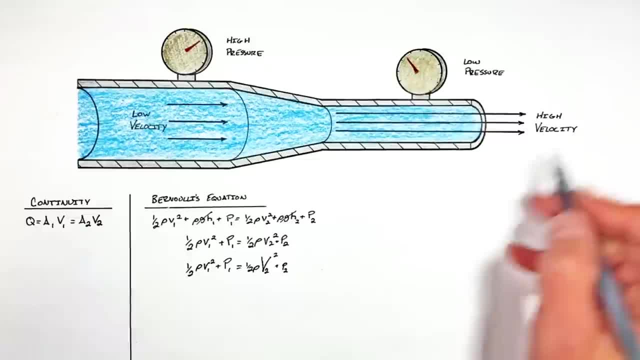 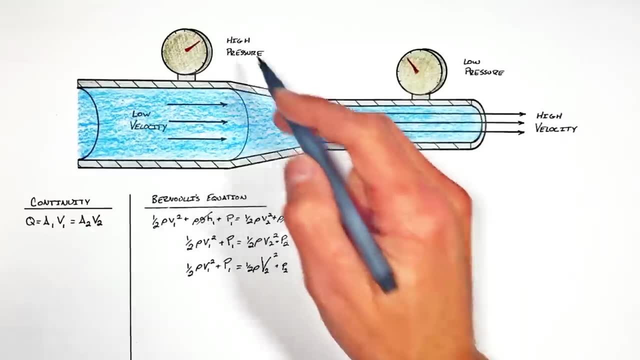 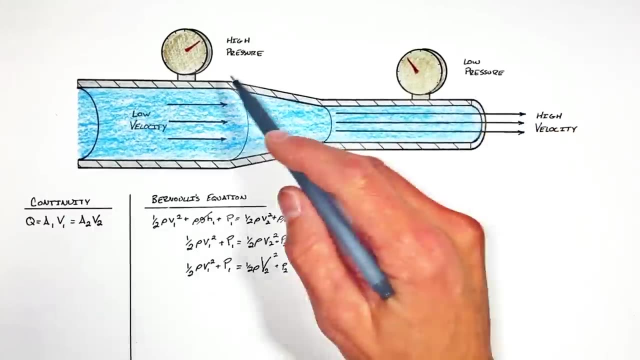 You see what I did there. Since I didn't have numbers, I just made a big V for higher velocity and a smaller P for lower pressure. I am quite the educator. But the issue in this change in pressure is that it isn't particularly intuitive, And so people wonder why, Why did that pressure? 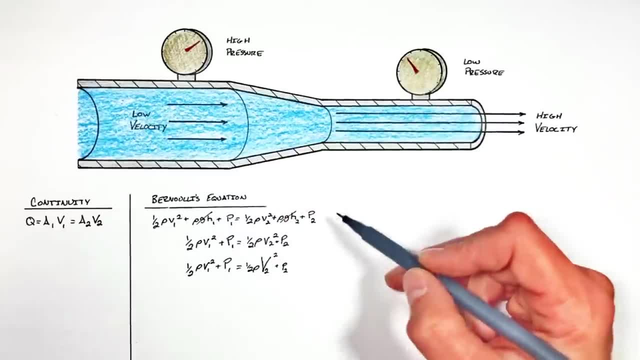 decrease in going through this pipe taper. Now people try to justify that change in pressure simply by referencing Bernoulli's equation And they say: well, if there's an increase in what we call the dynamic pressure, there must be a decrease in static pressure. Well, let's be honest, that's kind of a crap answer. 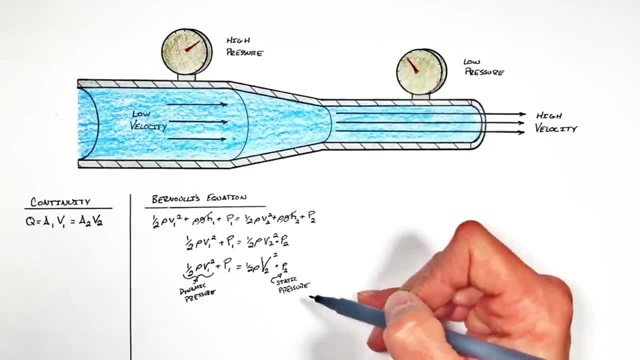 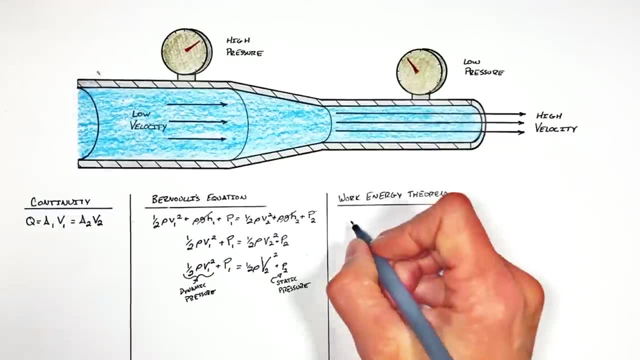 So how do we explain this change in pressure without using Bernoulli's equation? Now, the first place a lot of people are going to look is the work energy theorem. You see, the work energy theorem says that a change in kinetic energy of a particle is equal to the work. 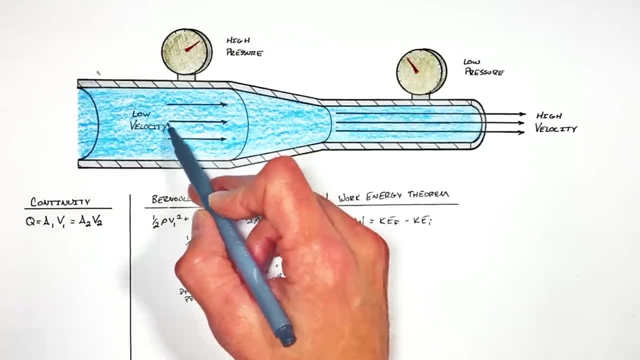 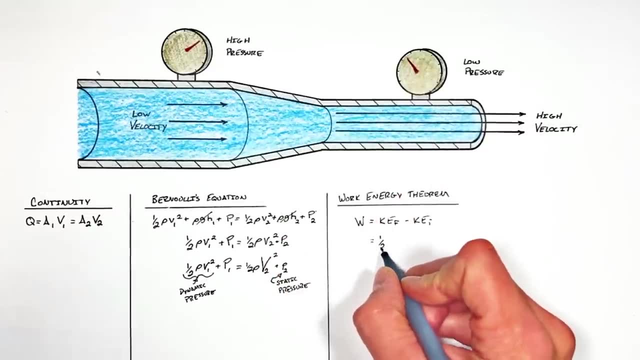 done on that particle. So if we were to look at an individual particle with some mass, as it moves from this position of low velocity to a higher velocity, That particle is going to have to have some increase in kinetic energy, Meaning there must be some work done on that. 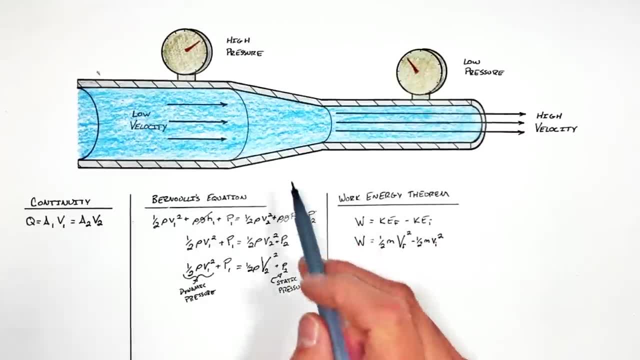 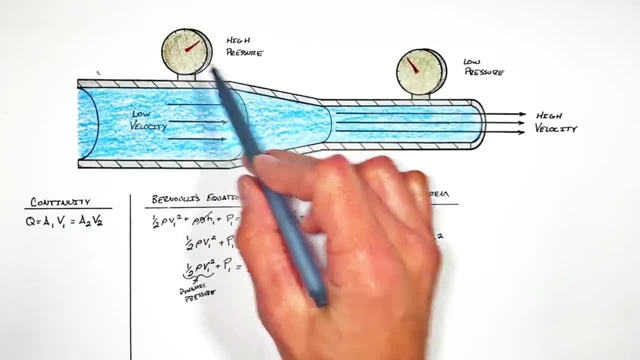 particle. So it's reasonable to justify that if there's been a work done on the particle, that energy had to come from somewhere and people attribute that work done to the drop in pressure. And again, while this isn't an incorrect explanation, it's really the same. 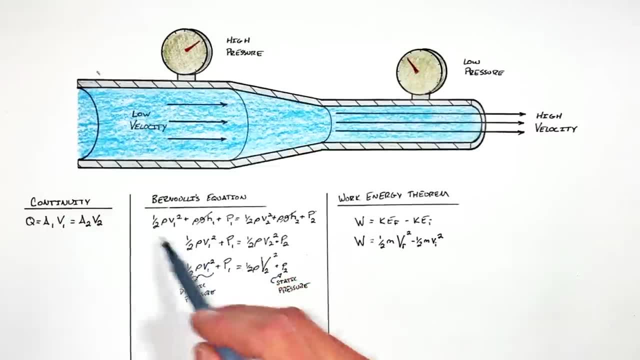 explanation: Bernoulli's equation. Remember Bernoulli's equation is derived directly from the work energy theorem. If you want to see that done, it's right here. which means both of these explanations really don't get at why the pressure decreases as the fluid goes from one pipe to. 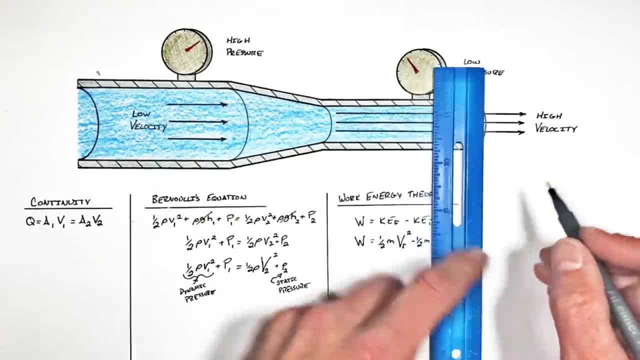 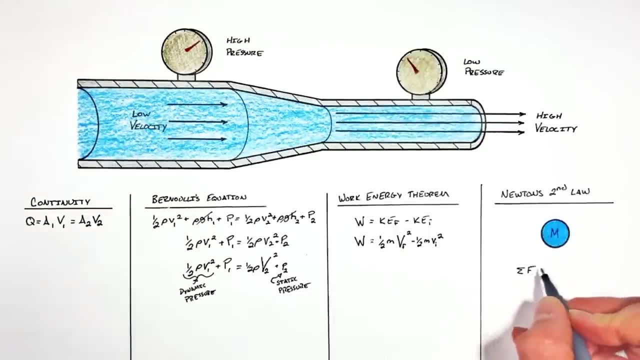 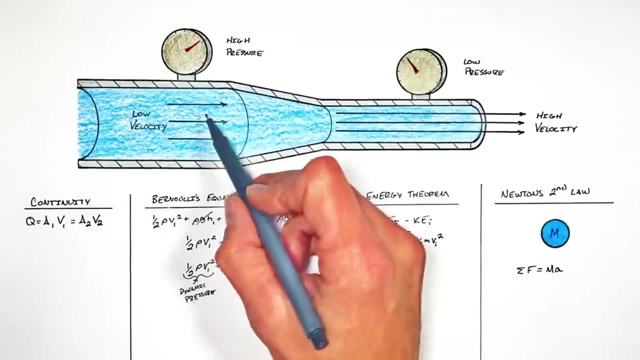 another. So let's back up to the very beginning of physics and take a look at Newton's second law Now. Newton's law says that sum of all forces is equal to mass times acceleration. So if we look at some mass or particle of fluid as it goes from a low velocity to a higher velocity, there must be 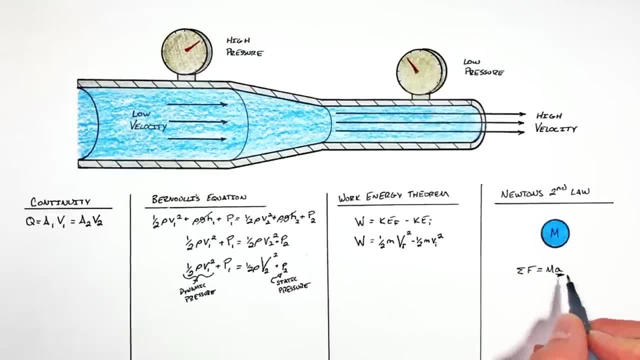 an acceleration of that particle. And if the particle accelerates, that means there must be some net force acting on that particle. Now there's pressure everywhere in this fluid pushing on every single particle. So if we look at some mass or particle of fluid, there must be some. 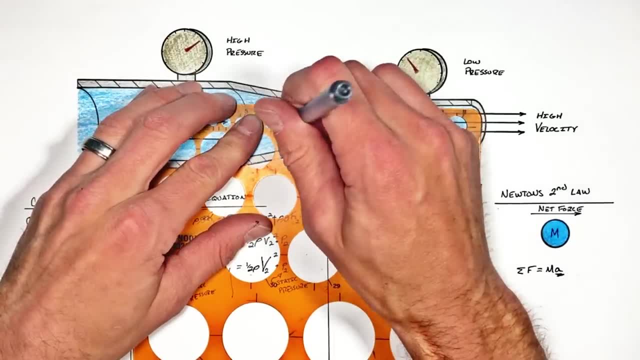 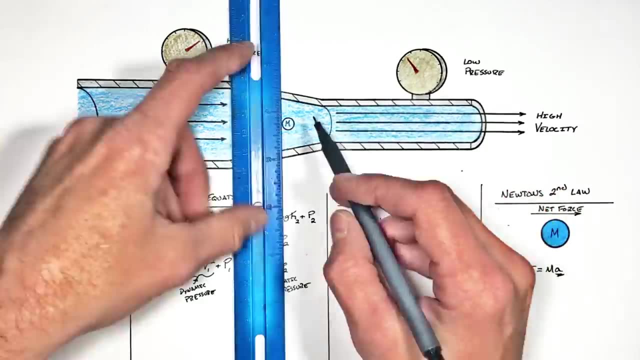 net force acting on that particle in every direction. But if we were to look at a particle right here which is accelerating as it goes from this large pipe to the smaller pipe, the pressure is not equal on this particle in every direction. And let me show you why. 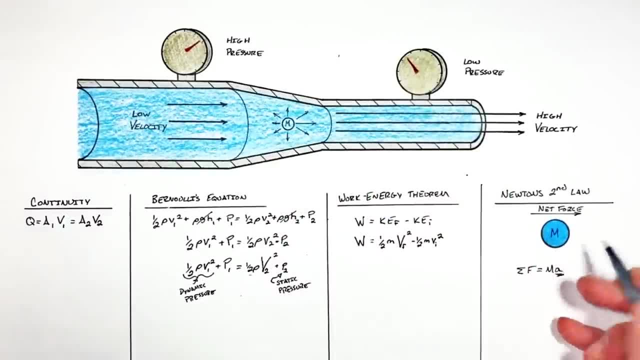 You see, if we look at this particle as though it's a free body diagram, in the horizontal axis there's going to be some force on this particle to the right, And that force is really from the pressure over the particle. So if we look at this particle as though it's a free body diagram, 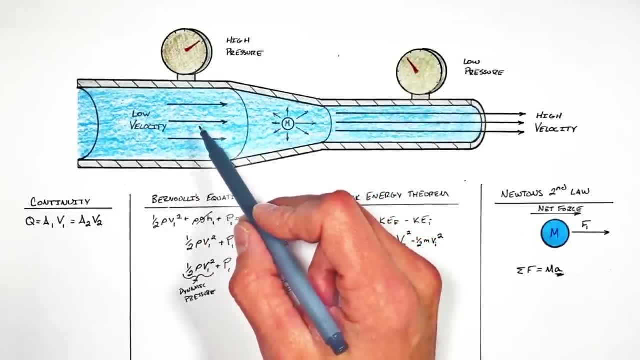 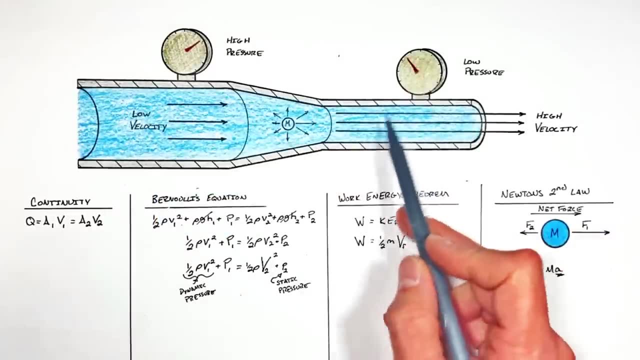 over here in the low velocity region of our flow. there's going to be a force horizontally to the left on this particle which is coming from the pressure over here in this higher velocity region And we know this force to the left has to be smaller than this force to the right. 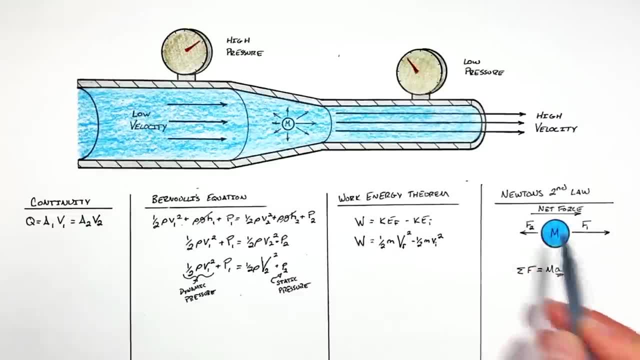 because we know there's a net force horizontally on this particle, causing it to accelerate as it goes from a large pipe to a smaller bore pipe. Now getting back to pressure, we know if a force acts on some particle, it's going to be a force that's going to be higher than this force to the 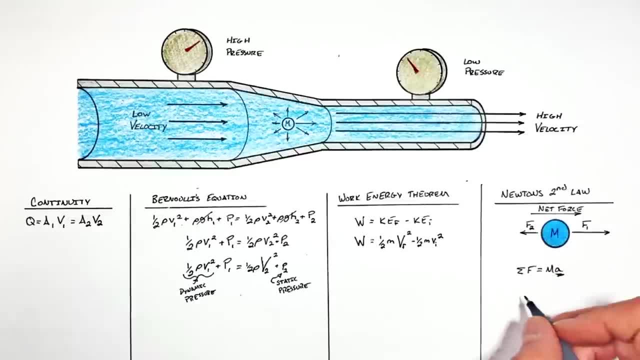 right. So if we look at this particle which has a certain cross-sectional area, which we'll call A, then the pressure on one side of the particle is going to be F1 over A And on the other side of the particle the pressure is going to be F2 over A And, since we know, F1 is larger than F2,. 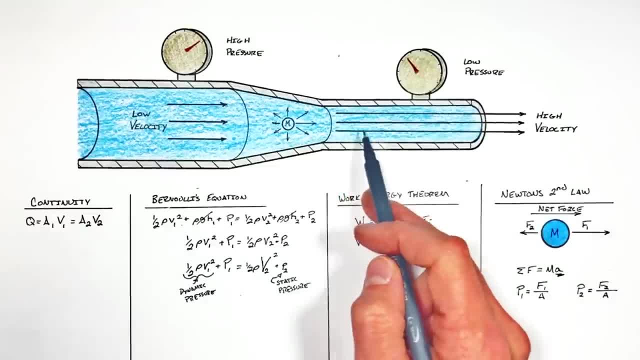 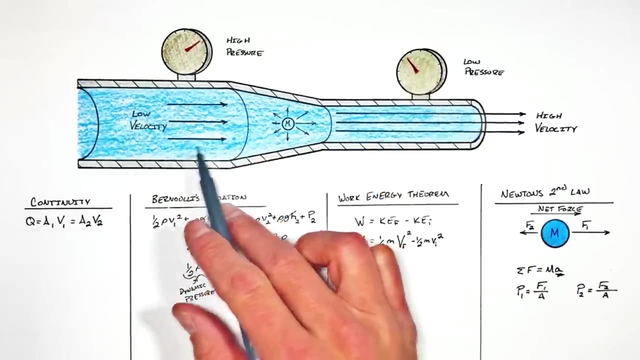 that means the pressure in the higher velocity region of this flow is going to be lower than in the lower velocity region of the flow, And there it is, in the most basic terms possible, the reasoning behind why the pressure decreases as fluid flows through this taper. Now it's important to point out here, if we allow a 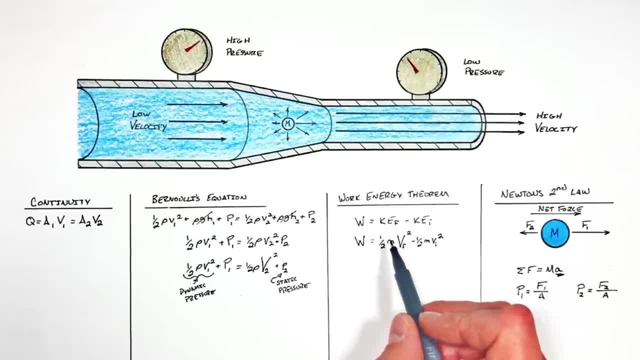 force to act over displacement. ultimately, what we now have is work, And if we substitute in fluid density rather than mass into the work energy theorem, what we wind up with is Bernoulli's equation. So realize, when somebody tries to justify this decrease in pressure using Bernoulli's 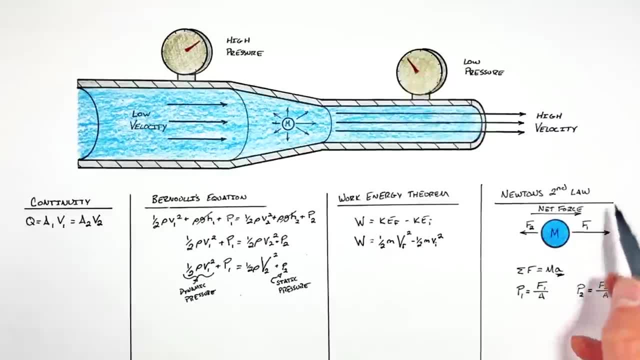 they're absolutely wrong. And so if we allow a force to act over displacement, ultimately what we correct. But if you dig down deep enough, it's really Newton's second law, or F equals MA, which is the true reasoning behind this decrease in pressure. So, Jesse Campbell and the rest of 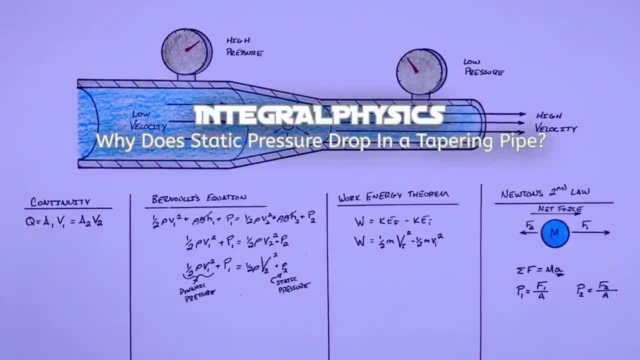 the internet. I hope you found this useful And, on that note, that's all for now.